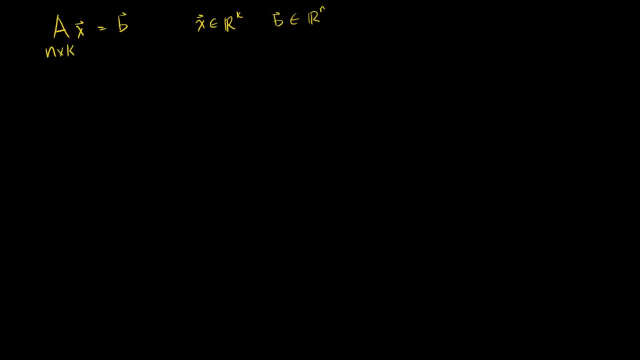 Now let's say that it just so happens that there is no solution to. AX is equal to B. What does that mean? Let's just expand out A. I think you already know what that means. If I write A like this: A1,, A2, if I just write it as its column vectors right there all the way through AK, and then I multiply it times X1,. 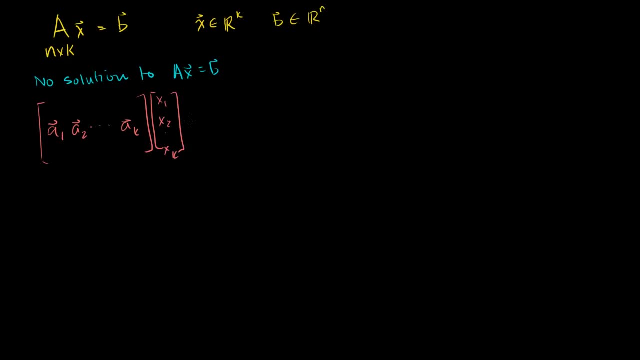 X2, all the way through XK. this is the same thing as that equation. there I just kind of wrote out the two matrices. Now this is the same thing as X1 times A1 plus X2 times A2, all the way to. plus XK times AK is equal to the vector B. 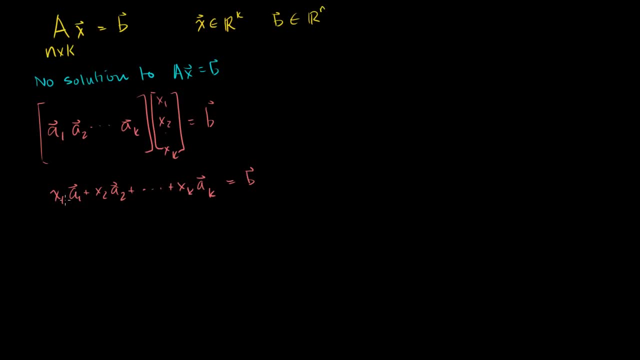 Now, if this has no solution, then that means that there's no set of weights here On the column vector B. there's no set of weights. There's no set of vectors of A where we can get to B, Or another way to say, it is no linear combinations of the column vectors of A will be equal to B. 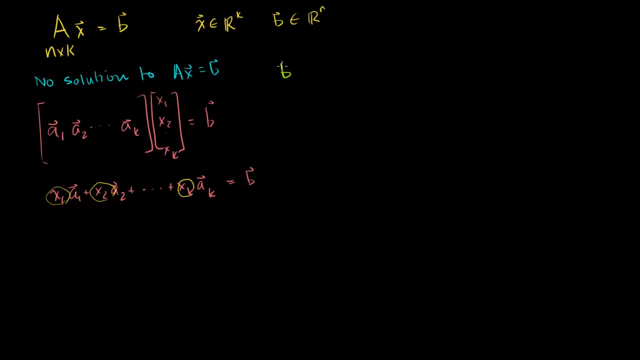 Or an even further way of saying it, is that B is not in the column space of A. No linear combination of these guys can equal to that, So let's see if we can visualize it a bit. So let me draw the column space of A. 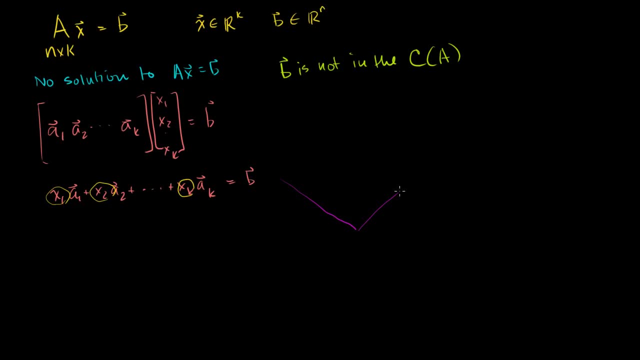 The column space of A looks something like this right here. I'll just assume it's a plane in Rn. It doesn't have to be a plane. Things can be very general, But let's say that this is the column space. This is the column space of A. 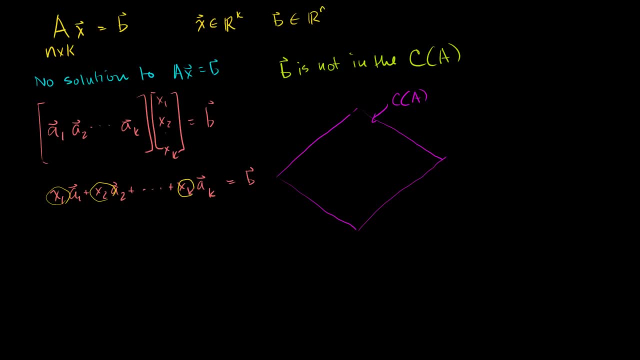 Now, if that's the column space and B is not in the column space, maybe we can draw B like this, Maybe B- let's say, this is the origin, right there, and B just pops out right there. So this is the zero vector. 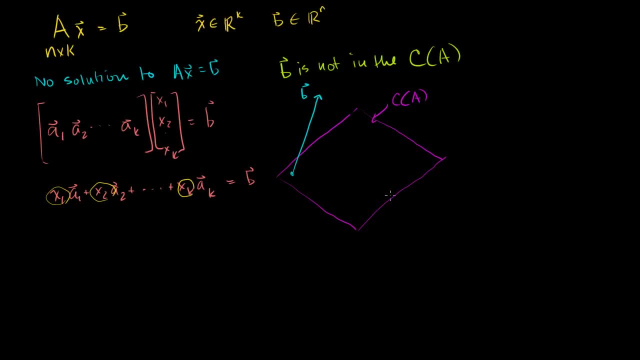 This is my vector B, Clearly not in my column space, It's clearly not in this plane. Now, up until now, we would get an equation like that. We would make an augmented matrix, put it in reduced row echelon form and get a line that said 0 equals 1.. 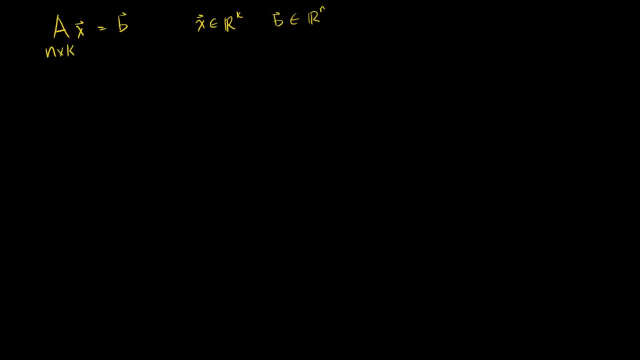 Now let's say that it just so happens that there is no solution to. AX is equal to B. What does that mean? Let's just expand out A. I think you already know what that means. If I write A like this: A1,, A2, if I just write it as its column vectors right there all the way through AK, and then I multiply it times X1,. 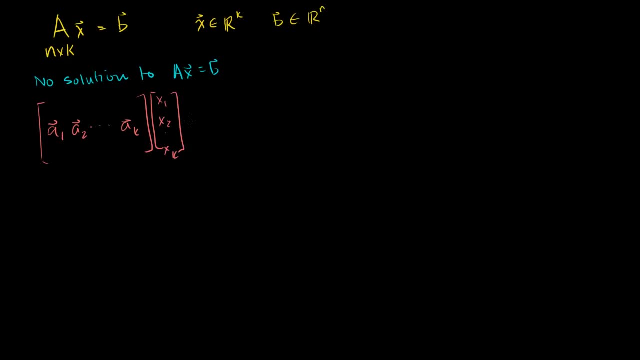 X2, all the way through XK. this is the same thing as that equation. there I just kind of wrote out the two matrices. Now this is the same thing as X1 times A1 plus X2 times A2, all the way to. plus XK times AK is equal to the vector B. 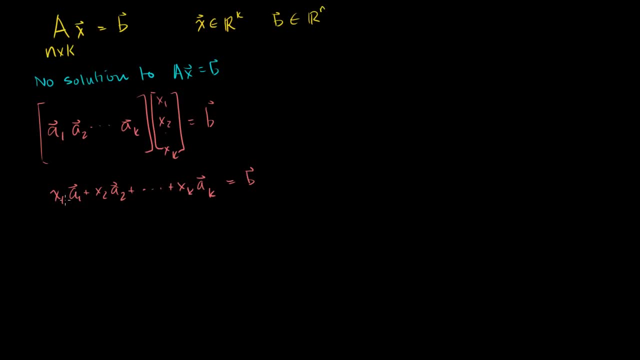 Now, if this has no solution, then that means that there's no set of weights here On the column vector B. there's no set of weights. There's no set of vectors of A where we can get to B, Or another way to say, it is no linear combinations of the column vectors of A will be equal to B. 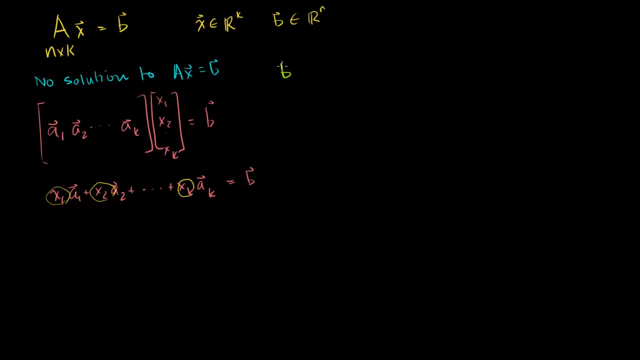 Or an even further way of saying it, is that B is not in the column space of A. No linear combination of these guys can equal to that, So let's see if we can visualize it a bit. So let me draw the column space of A. 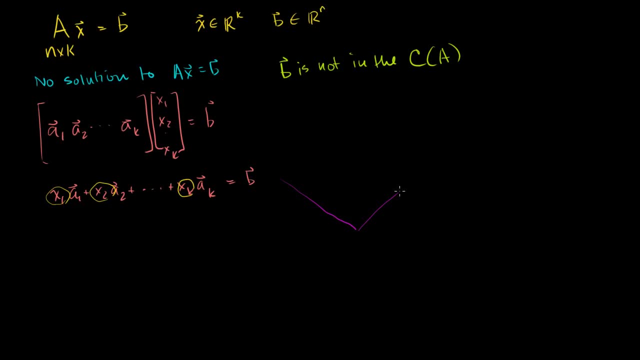 The column space of A looks something like this right here. I'll just assume it's a plane in Rn. It doesn't have to be a plane. Things can be very general, But let's say that this is the column space. This is the column space of A. 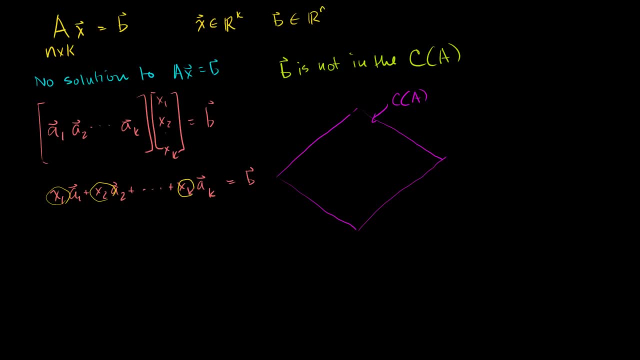 Now, if that's the column space and B is not in the column space, maybe we can draw B like this, Maybe B- let's say, this is the origin, right there, and B just pops out right there. So this is the zero vector. 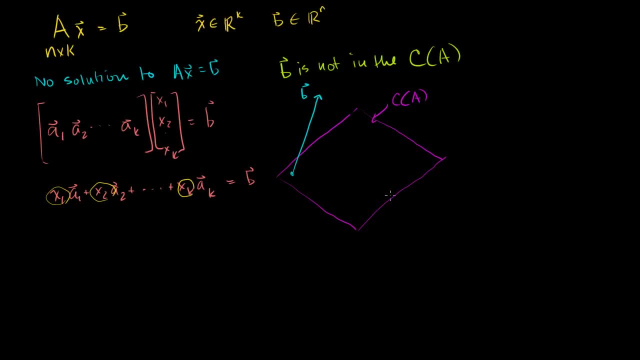 This is my vector B, Clearly not in my column space, It's clearly not in this plane. Now, up until now, we would get an equation like that. We would make an augmented matrix, put it in reduced row echelon form and get a line that said 0 equals 1.. 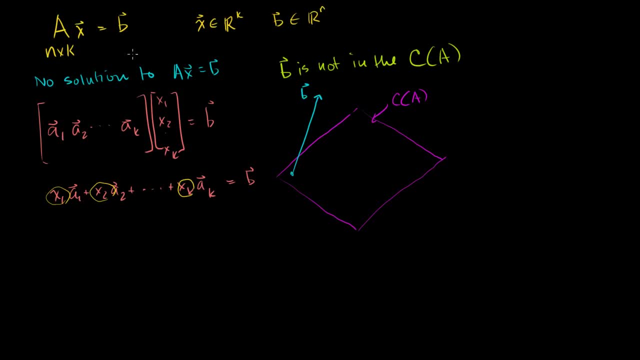 And we'd say: no solution, nothing we can do here. But what if we can do better? We clearly can't find a solution to this, But what if we can find a solution that gets us close to this? So what if I want to find some x. 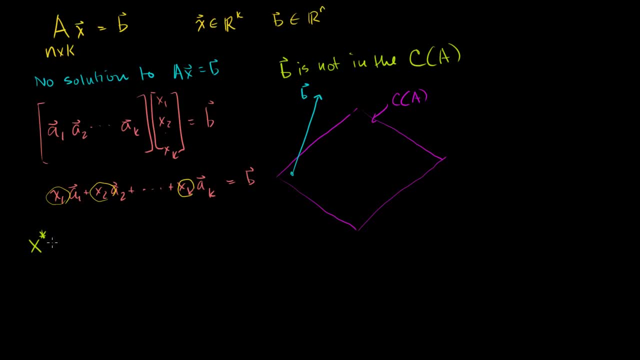 I'll call it x star For now. So I want to find some x star where A times x star is- and this is a vector- is as close as possible. Let me write this As close to B as possible, Or another way to view it. when I say close, I'm talking about length. 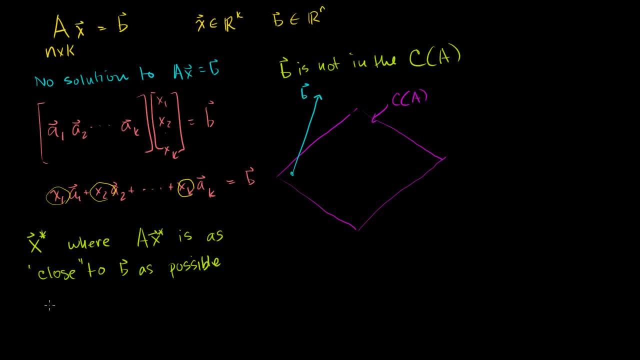 I want to minimize the length of. let me write this down: I want to minimize the length of B minus A times x star. Now some of y'all might already know where this is going, But when you take the difference between two and then take its length, what does that look like? 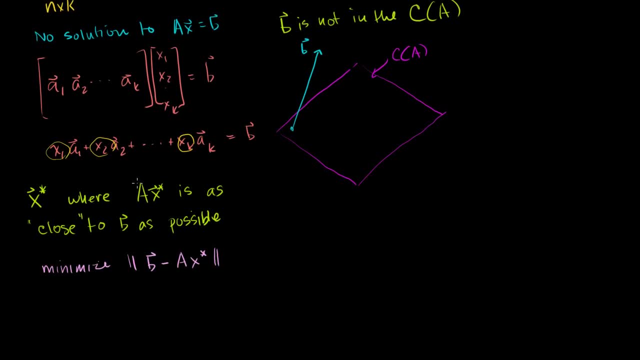 What does that look like? Let me just call A x. A x is going to be a member of my column space. Let me just call that V. A x is equal to V, Since we're taking some linear. you multiply any vector in RK times the columns of times your matrix A. 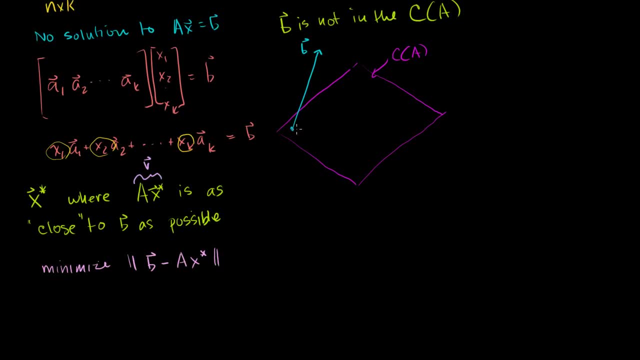 you're going to get a member of your column space. So any A x is going to be is going to be in your column space. So any A x is going to be in your column space, And maybe that is. the vector of V is equal to A times. 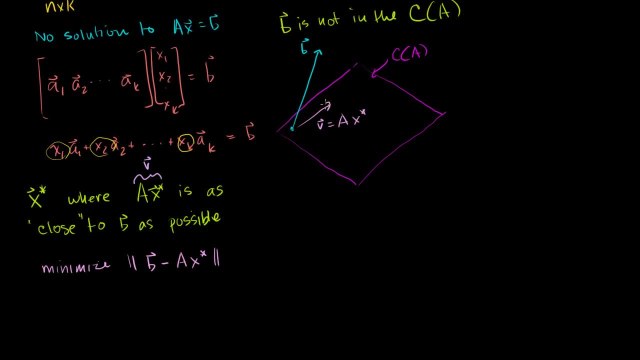 vector of V is equal to A times x star. We want this vector to get as close as possible to this, as as long as it stays- I mean, it has to be in my column space, But we want this- the distance between this vector and this vector- to be minimized. 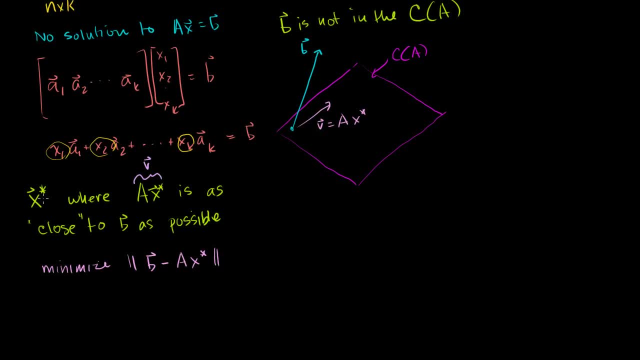 Now I just want to show you where the terminology for this will come from. I haven't given it its proper title yet. If you were to take this vector, I'm saying that this is: let's just call this vector V for simplicity. 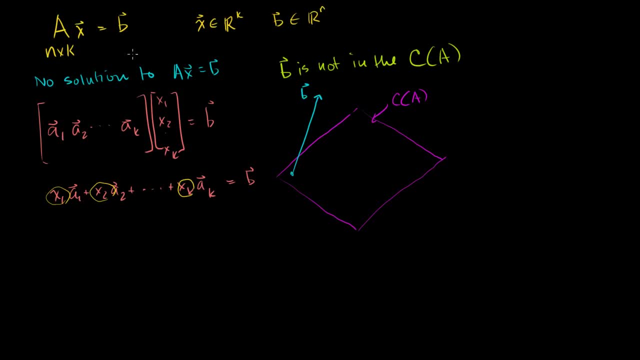 And we'd say: no solution, nothing we can do here. But what if we can do better? We clearly can't find a solution to this, But what if we can find a solution that gets us close to this? So what if I want to find some x. 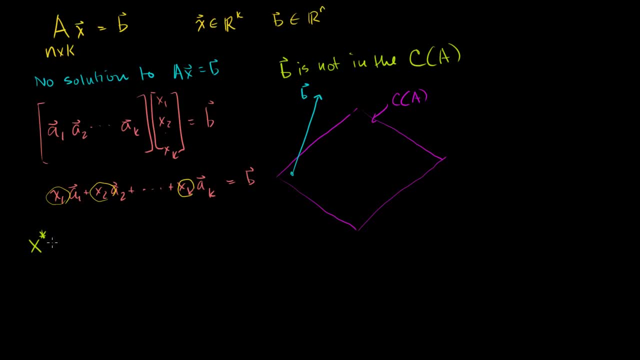 I'll call it x star For now. So I want to find some x star where A times x star is- and this is a vector- is as close as possible. Let me write this As close to B as possible, Or another way to view it. when I say close, I'm talking about length. 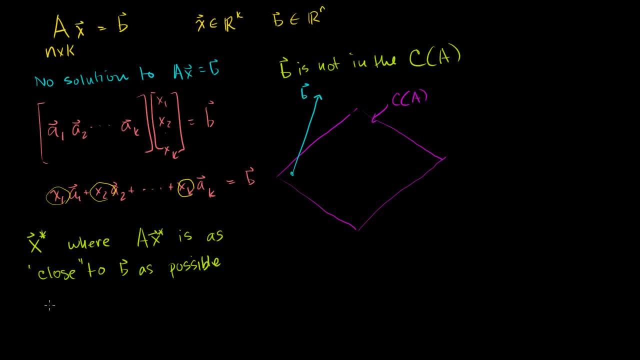 I want to minimize the length of. let me write this down: I want to minimize the length of B minus A times x star. Now some of y'all might already know where this is going, But when you take the difference between two and then take its length, what does that look like? 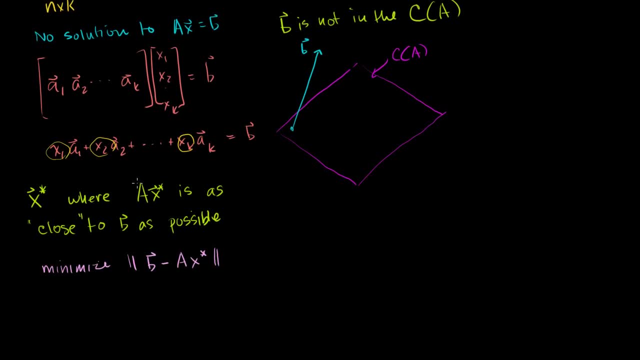 What does that look like? Let me just call A x. A x is going to be a member of my column space. Let me just call that V. A x is equal to V, Since we're taking some linear. you multiply any vector in RK times the columns of times your matrix A. 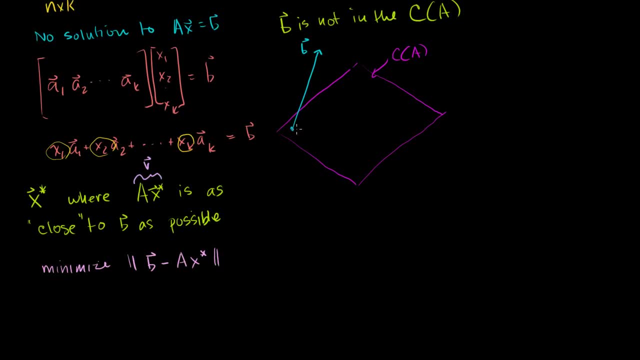 you're going to get a member of your column space. So any A x is going to be is going to be in your column space. So any A x is going to be in your column space, And maybe that is. the vector of V is equal to A times. 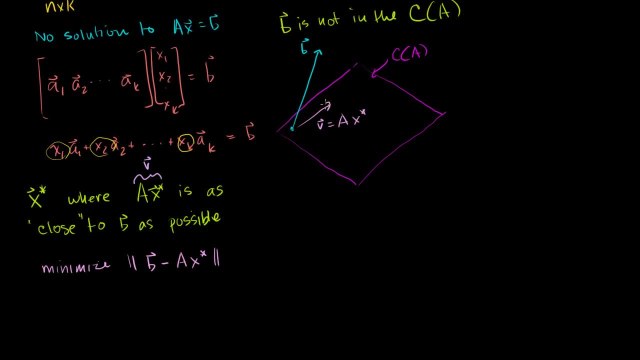 vector of V is equal to A times x star. We want this vector to get as close as possible to this, as as long as it stays- I mean, it has to be in my column space, But we want this- the distance between this vector and this vector- to be minimized. 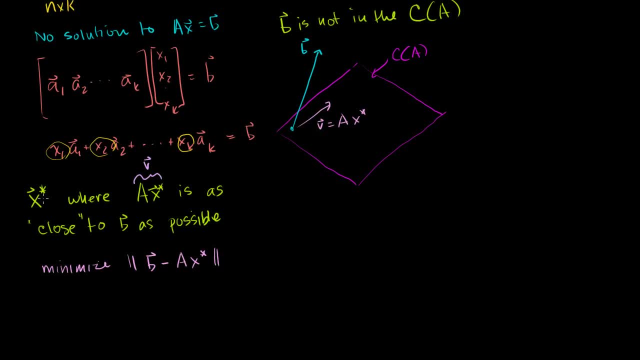 Now I just want to show you where the terminology for this will come from. I haven't given it its proper title yet. If you were to take this vector, I'm saying that this is: let's just call this vector V for simplicity. 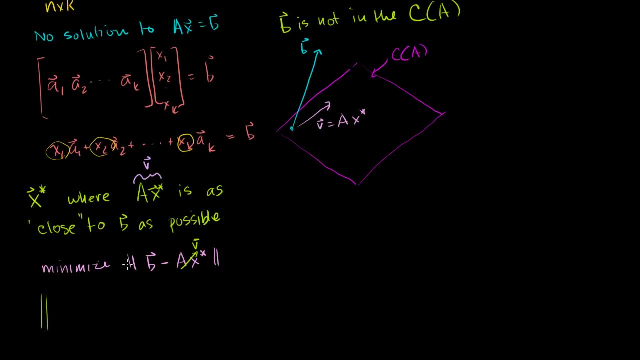 This is equivalent to the length of the vector, of the vector. you take the difference between each of the elements, So b1 minus v1,, b2 minus v2, all the way to bn minus vn. And if you take the length of this vector, 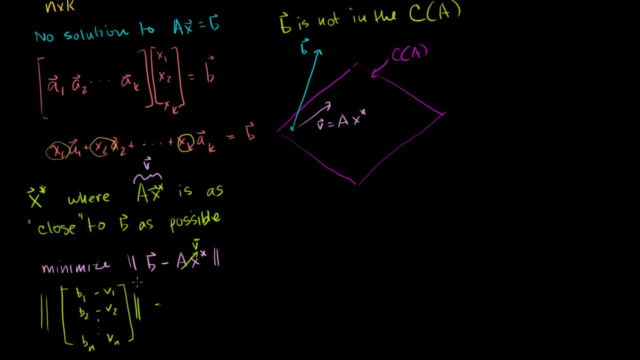 this is the same thing as this. this is going to be equal to the square root. Let me take the length squared. actually, The length squared of this is just going to be b1 minus v1 squared plus b2 minus v2.. 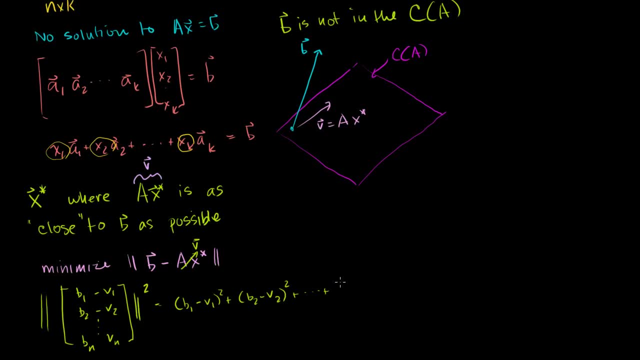 minus v2 squared, plus all the way to bn minus vn squared, And I want to minimize this. So I want to make this value the least value that it can be possible. I want to get the least squares estimate here, And that's why. 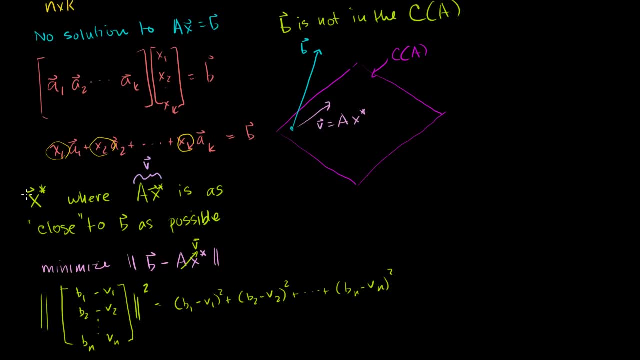 this last minute or two when I was just explaining this. that was just to give you the motivation for why this right here is called the least squares estimate, Least squares estimate, Or the least squares solution, or the least squares approximation for the equation ax equals b. 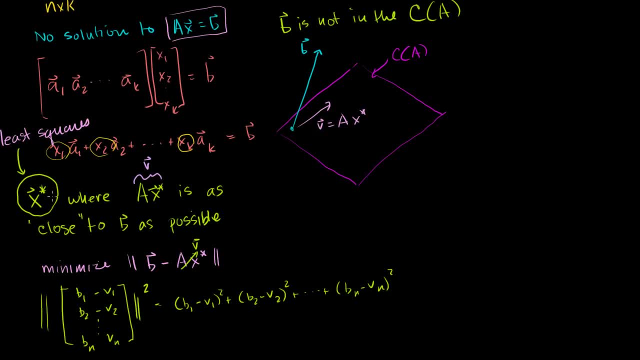 There is no solution to this, But maybe we can find some x star where, if I multiply a times x star, this is clearly going to be in my column space and I want to get this vector to be as close to b as possible. 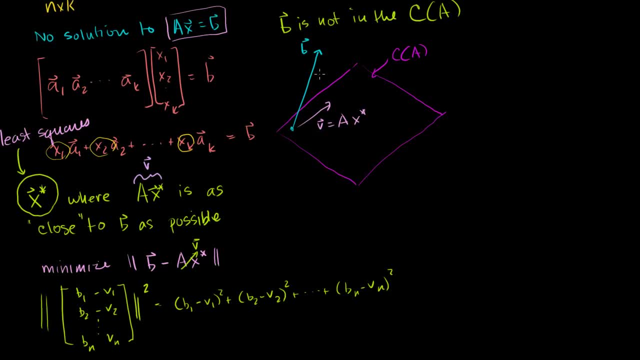 Now we've already seen in several videos what is the closest vector in any subspace to a vector that's not in my subspace. Well, the closest vector to it is the projection. The closest vector to b that's in my subspace. 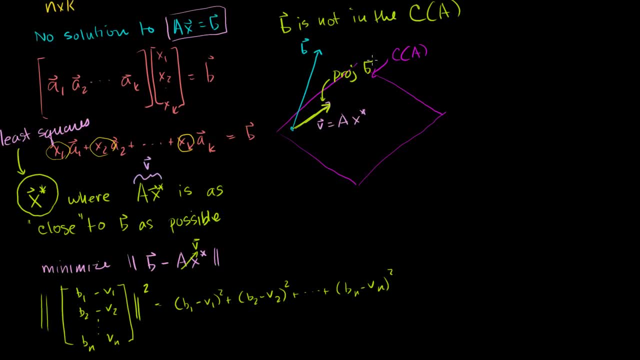 is going to be the projection of b onto my column space. That is the closest vector there. So if I want to minimize this, I'm essentially I want to figure out my x star, where ax star is equal to the projection of my vector b. 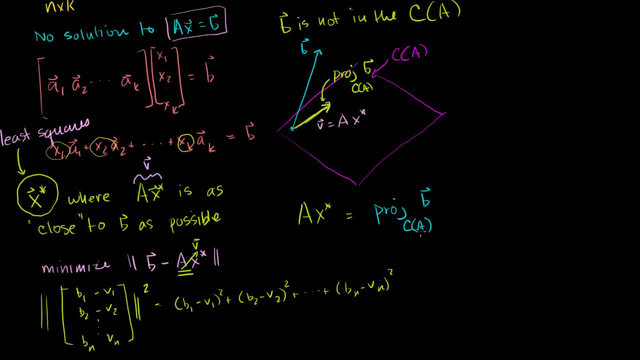 onto my subspace or onto the column space of a. Remember what we're doing here. We said axb has no solution, But maybe we can find some x that gets us as close as possible, So that I'm calling that my least squares solution. 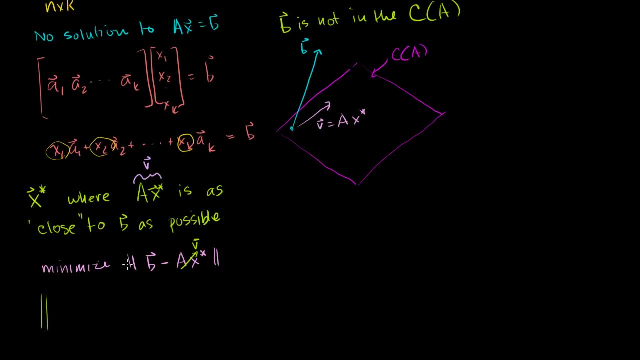 This is equivalent to the length of the vector, of the vector. you take the difference between each of the elements, So b1 minus v1,, b2 minus v2, all the way to bn minus vn. And if you take the length of this vector, 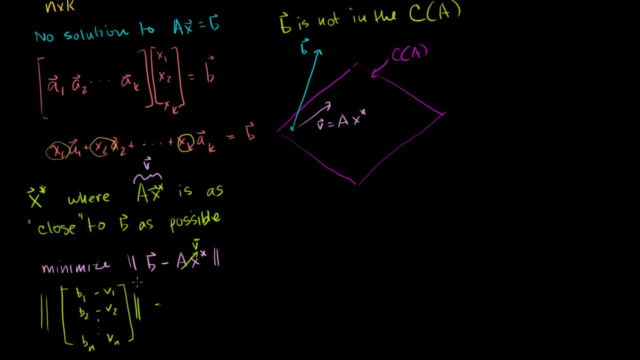 this is the same thing as this. this is going to be equal to the square root. Let me take the length squared. actually, The length squared of this is just going to be b1 minus v1 squared plus b2 minus v2.. 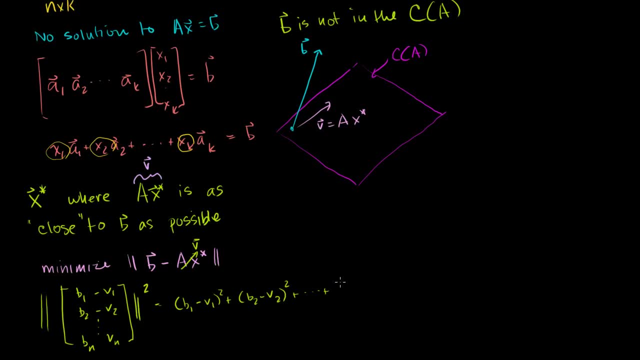 minus v2 squared, plus all the way to bn minus vn squared, And I want to minimize this. So I want to make this value the least value that it can be possible. I want to get the least squares estimate here, And that's why. 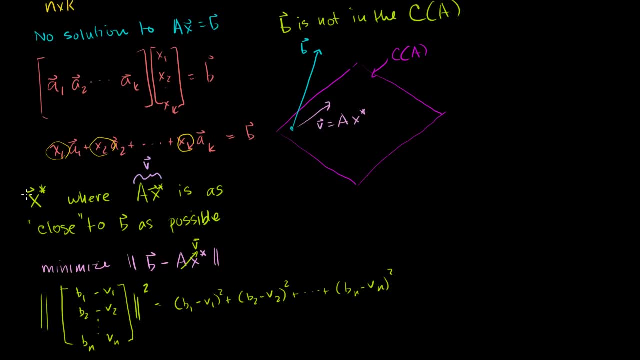 this last minute or two when I was just explaining this. that was just to give you the motivation for why this right here is called the least squares estimate, Least squares estimate, Or the least squares solution, or the least squares approximation for the equation ax equals b. 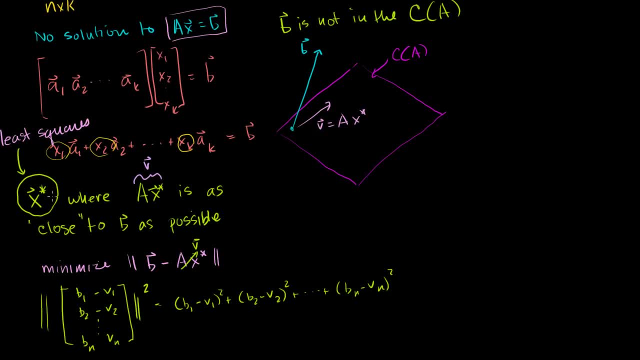 There is no solution to this, But maybe we can find some x star where, if I multiply a times x star, this is clearly going to be in my column space and I want to get this vector to be as close to b as possible. 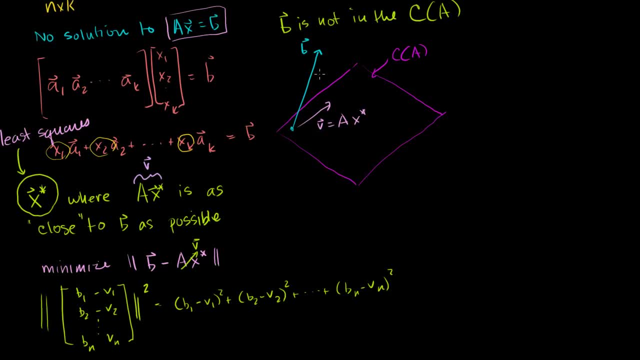 Now we've already seen in several videos what is the closest vector in any subspace to a vector that's not in my subspace. Well, the closest vector to it is the projection. The closest vector to b that's in my subspace. 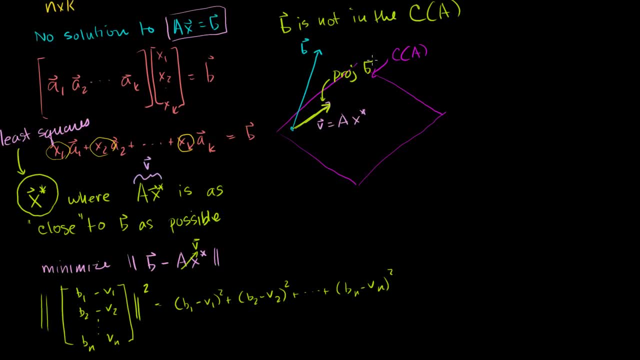 is going to be the projection of b onto my column space. That is the closest vector there. So if I want to minimize this, I'm essentially I want to figure out my x star, where ax star is equal to the projection of my vector b. 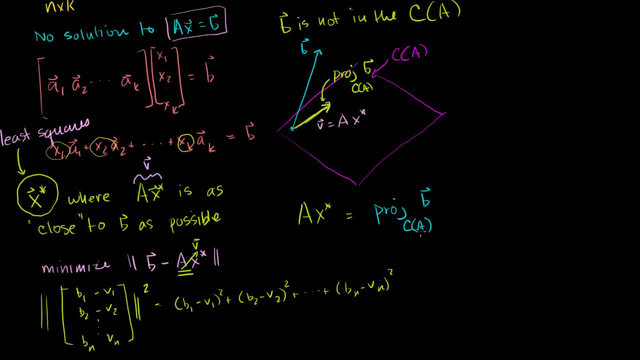 onto my subspace or onto the column space of a. Remember what we're doing here. We said axb has no solution, But maybe we can find some x that gets us as close as possible, So that I'm calling that my least squares solution. 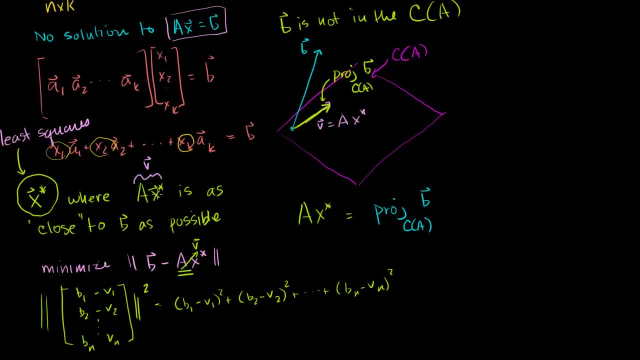 Or my least squares, approximation. And this guy right here is clearly going to be in my column space, Right, Because you take some vector x times a. that's going to be a linear combination of these column vectors, So it's going to be in the column space. 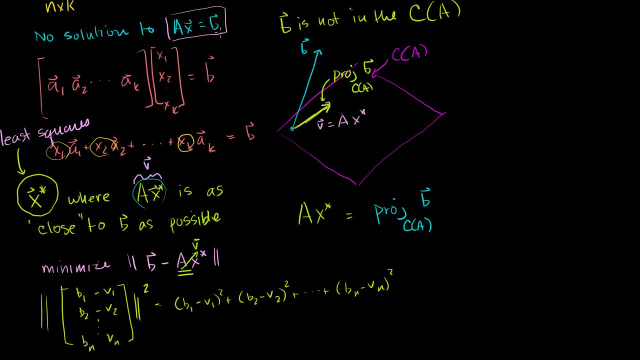 And I want this guy to be as close as possible to this guy. To be as close as possible to that guy. Well, the closest vector in my column space to that guy is the projection. So I want: so ax needs to be equal to the projection of b. 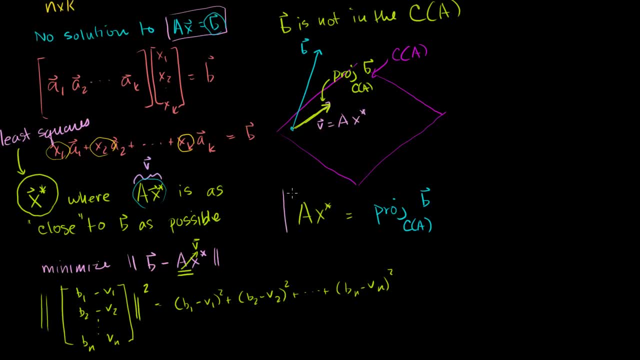 on my column space. It needs to be equal to that. But this is still pretty hard to find. you know, to find that. you saw how you know you took a times the inverse of a transpose, a times a transpose. It's hard to find that transformation matrix. 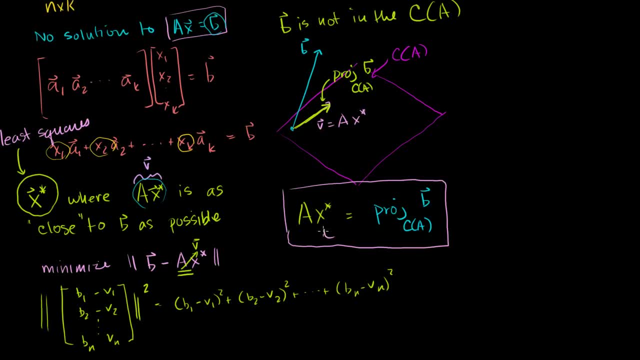 So let's see if we can find an easier way to figure out the least squares solution Or kind of our best solution. It's not the solution, It's our best solution to this right here, And that's what we call the least squares solution or approximation. 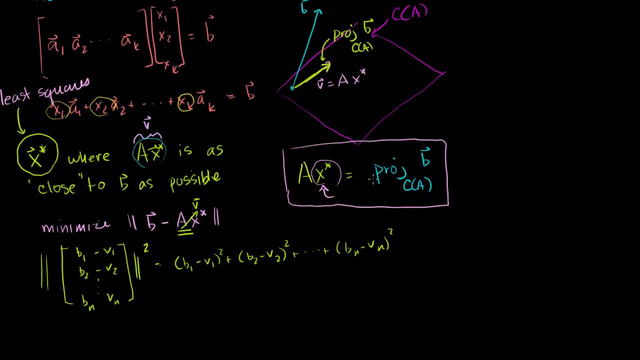 So if we let's just subtract b from both sides of this and we'll, we might get something interesting. So what happens if we, if we take ax minus the vector b on both sides of this equation? I'll do it up here in the right. 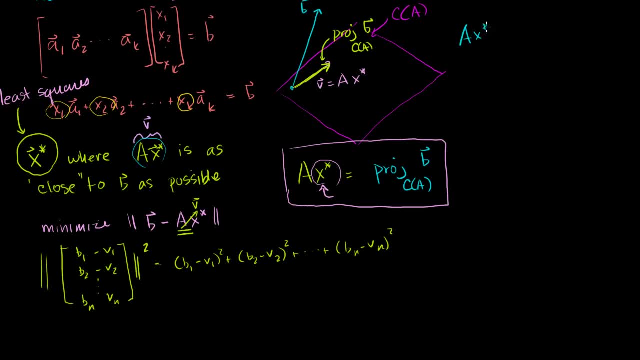 So if we on the left hand side we get a times x star, It's hard to write the x and then the star because they're very similar. And then we subtract b from it, We subtract our vector b, That's going to be equal to: 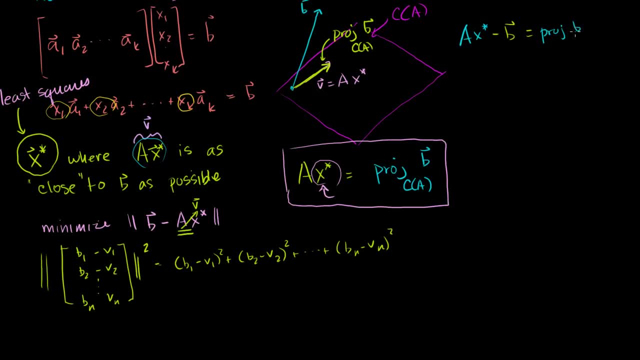 the projection, the projection of b onto our column space minus b. All I did is I subtracted b from both sides of this equation. Now, what is the projection of b minus our vector b? If we draw it right here, it's going to be this vector, right. 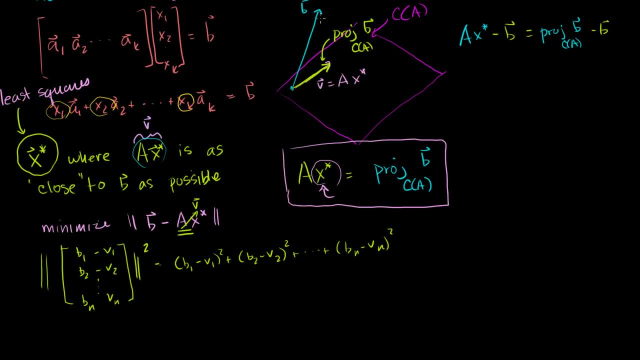 Let me do it in. let me do it in this orange color. It's going to be this, right here. It's going to be that vector, right there, Right. If I take the projection of b, which is that minus b, 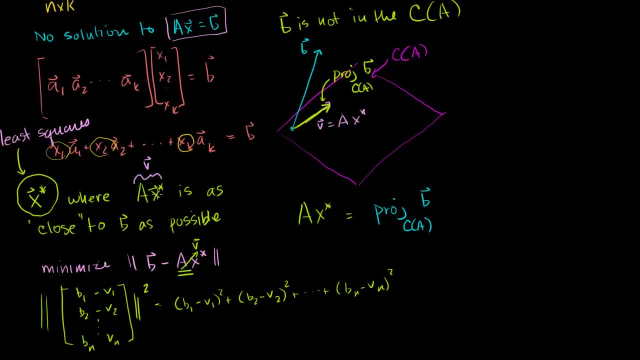 Or my least squares, approximation. And this guy right here is clearly going to be in my column space, Right, Because you take some vector x times a. that's going to be a linear combination of these column vectors, So it's going to be in the column space. 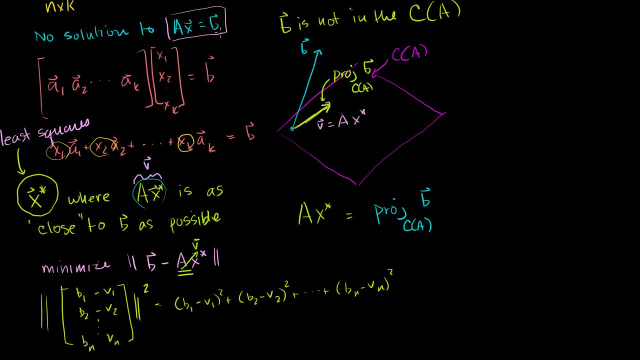 And I want this guy to be as close as possible to this guy. To be as close as possible to that guy. Well, the closest vector in my column space to that guy is the projection. So I want: so ax needs to be equal to the projection of b. 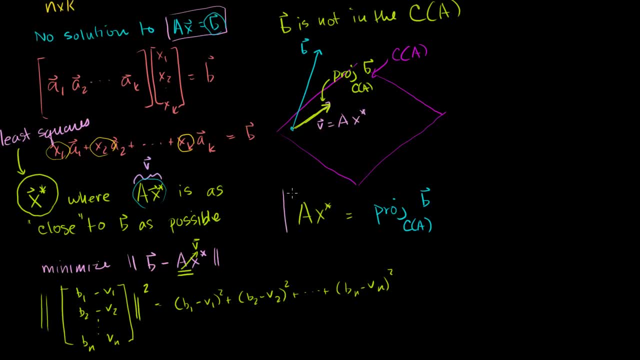 on my column space. It needs to be equal to that. But this is still pretty hard to find. you know, to find that. you saw how you know you took a times the inverse of a transpose, a times a transpose. It's hard to find that transformation matrix. 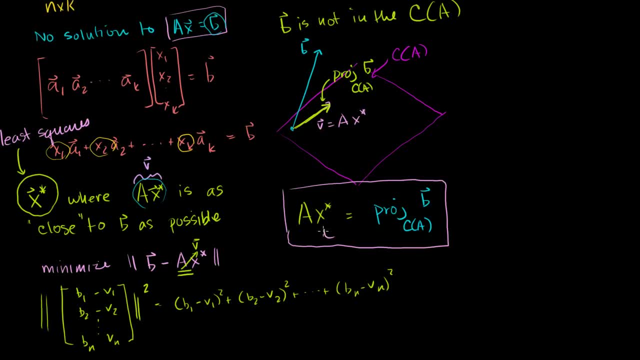 So let's see if we can find an easier way to figure out the least squares solution Or kind of our best solution. It's not the solution, It's our best solution to this right here, And that's what we call the least squares solution or approximation. 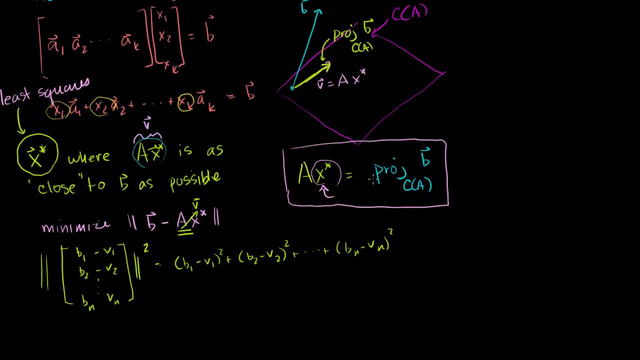 So if we let's just subtract b from both sides of this and we'll, we might get something interesting. So what happens if we, if we take ax minus the vector b on both sides of this equation? I'll do it up here on the right. 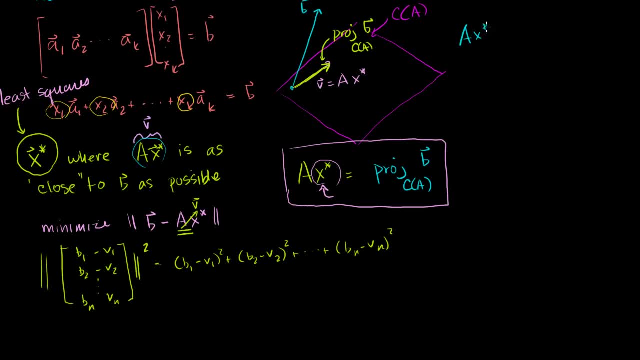 So if we on the left hand side we get a times x star, It's hard to write the x and then the star because they're very similar. And then we subtract b from it, We subtract our vector b, That's going to be equal to: 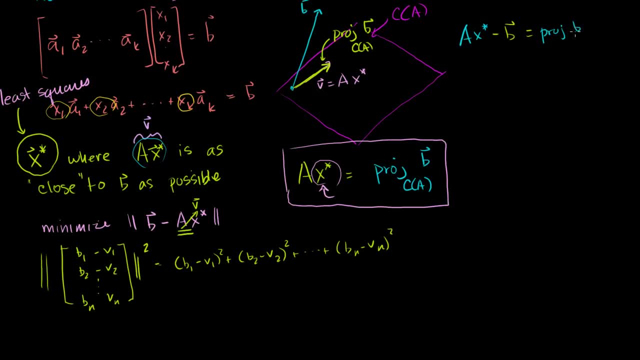 the projection, the projection of b onto our column space minus b. All I did is I subtracted b from both sides of this equation. Now, what is the projection of b minus our vector b? If we draw it right here, it's going to be this vector, right. 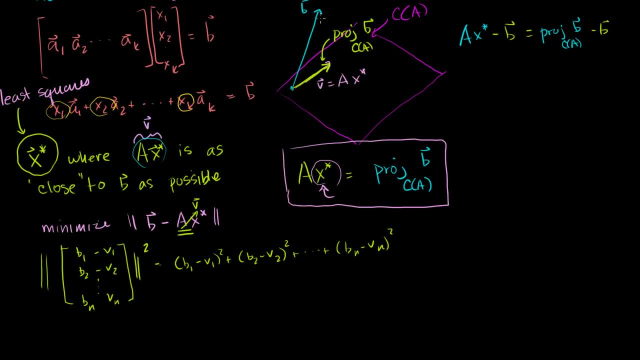 Let me do it in. let me do it in this orange color. It's going to be this, right here. It's going to be that vector, right there, right. If I take the projection of b, which is that minus b, 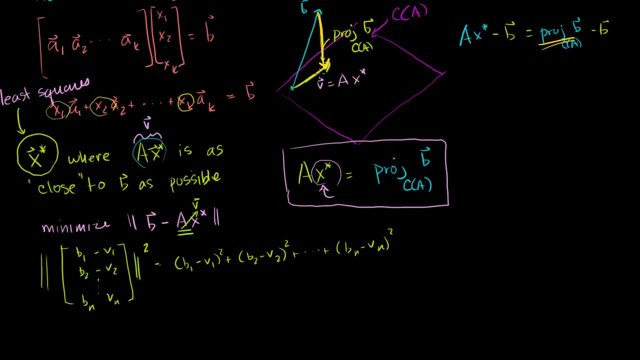 I'm going to get this vector. You can say b plus this vector is equal to my projection of b onto my subspace. So this vector right here is orthogonal. It's actually part of the definition of a projection That this guy, this guy, is going to be orthogonal. 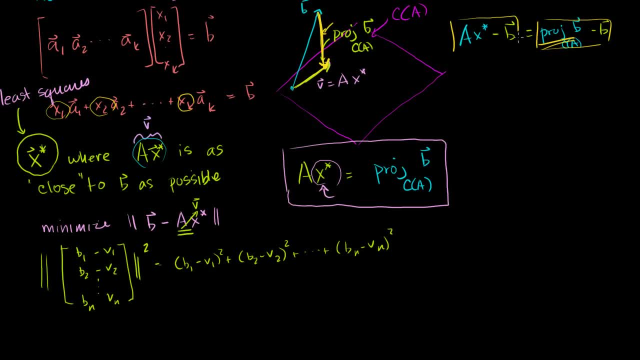 to my subspace or to my column space, And so this guy is orthogonal to my column space. Right, I can write ax star minus b: It's orthogonal to my column space. or we could say it's a member of the orthogonal complement of my column space. 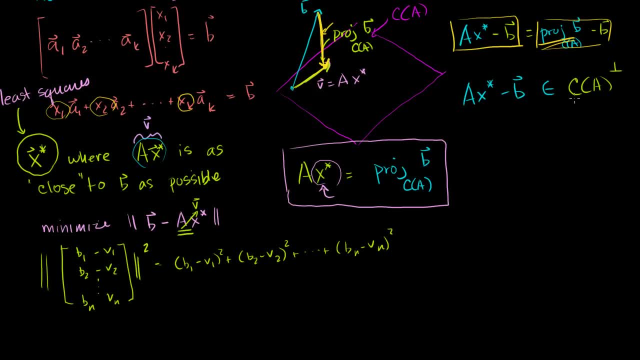 Right, The orthogonal complement is just the set of everything. the set of everything, all of the vectors that are orthogonal to everything in your subspace, in your column space, right here. So this, this vector, right here, this kind of pointing straight down. 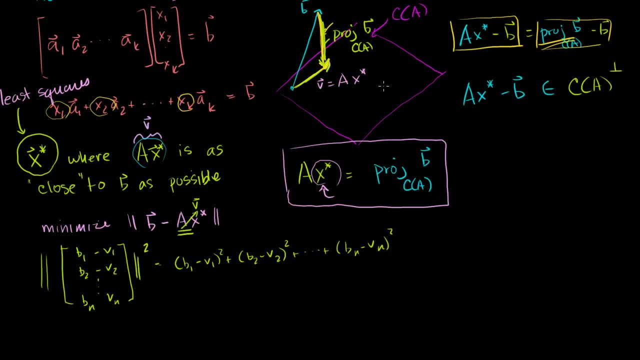 to my plane is clearly a member of the orthogonal complement of my column space. Now we've this might look familiar to you already. What is the orthogonal complement of my column space? The orthogonal complement of my column space is equal to the null space. 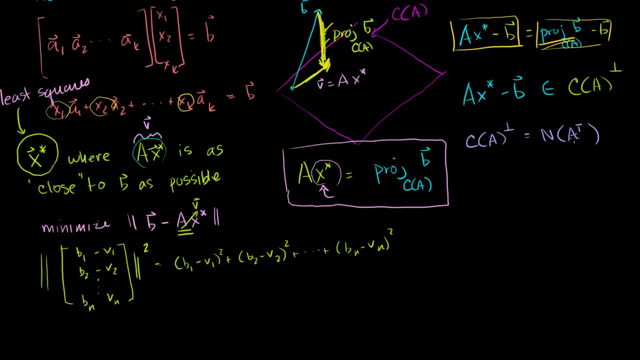 of A, transpose Right Or the left null space of A. We've done this in many, many videos So we can say: we can say that A times my least squares estimate of the equation AX is equal to B. I wrote that. 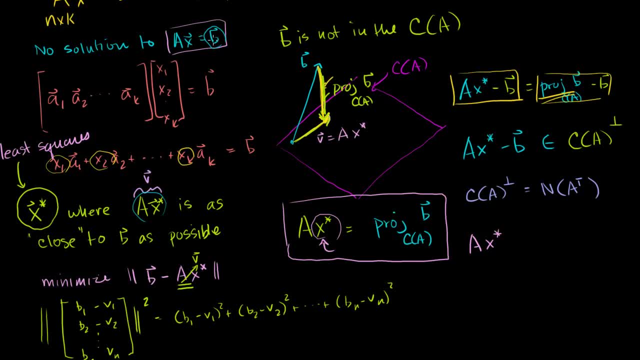 So X star is my least squares solution to AX is equal to B. So A times that minus B, minus B is a member of the null space of A transpose. Now, what does that mean? Well, that means that if I multiply A transpose: 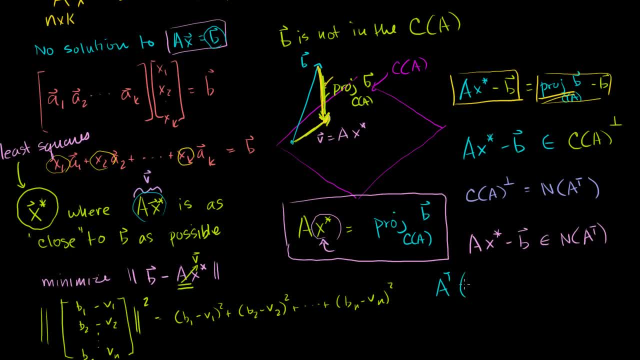 if I multiply A, transpose times, this guy right here times AX star. and let me, I don't want to lose the vector signs there on the X. This is a vector, Don't want to forget that. AX star minus B. 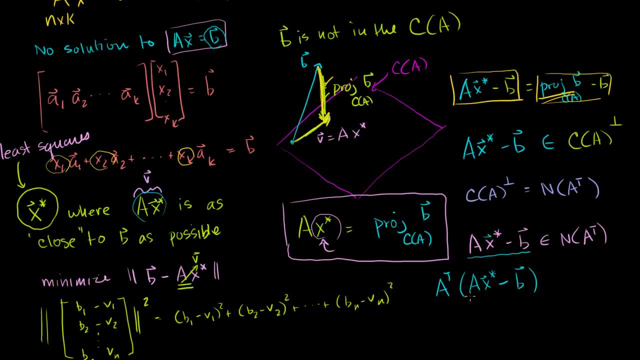 So if I multiply A transpose times this, right there, that is the same thing as that. What am I going to get? Well, this is a member of the null space of A transpose, So this times A transpose has got to be equal to zero. 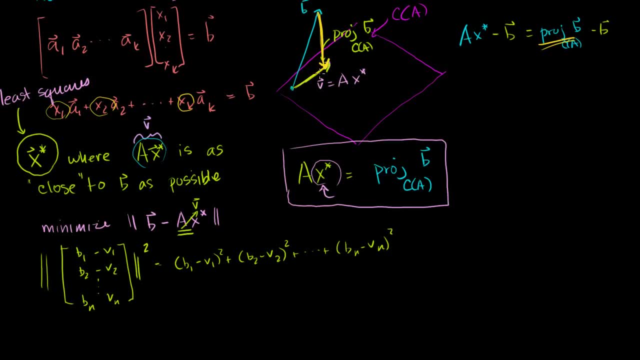 I'm going to get this vector. You could say b plus this vector is equal to my projection of b onto my subspace. So this vector right here is orthogonal. It's actually part of the definition of a projection That this guy, this guy, is going to be orthogonal. 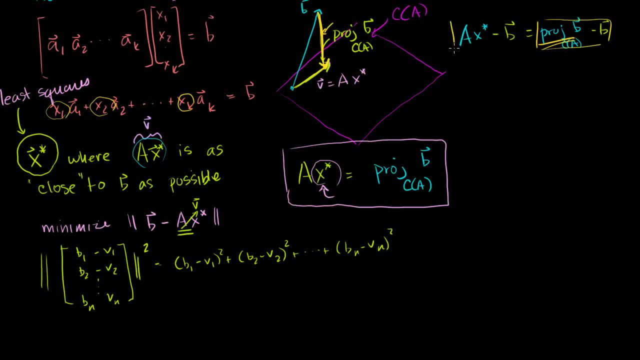 to my subspace or to my column space, And so this guy is orthogonal to my column space. So I could write: I can write ax, star minus b, It's orthogonal to my column space. or we could say it's a member of the orthogonal complement of my column space. 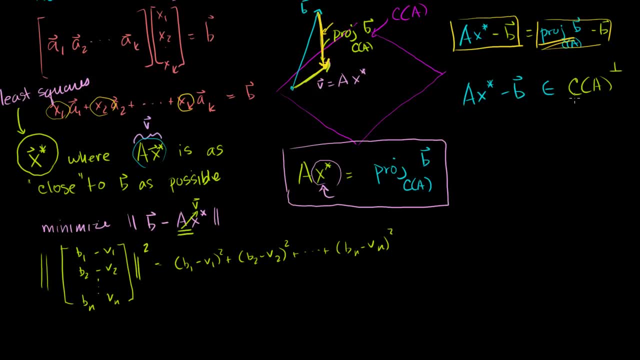 Right, The orthogonal complement is just the set of everything. the set of everything, all of the vectors that are orthogonal to everything in your subspace, in your column space, right here. So this, this vector, right here, this kind of pointing straight down onto my plane. 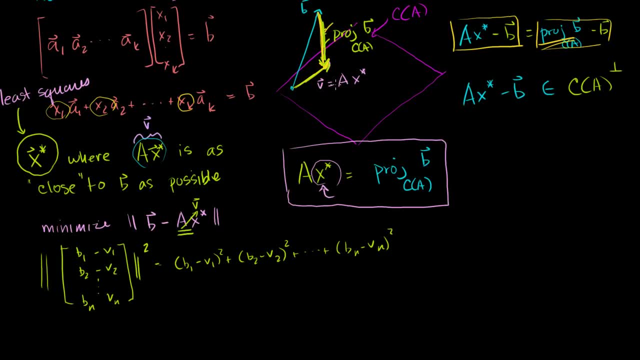 is clearly a member of the orthogonal complement of my column space. Now we've this might look familiar to you already. What is the orthogonal complement of my column space? The orthogonal complement of my column space is equal to the null space of a transpose. 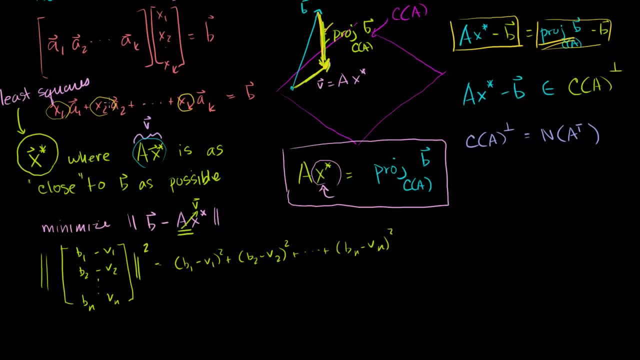 Right Or the left. null space of a. We've done this in many, many videos, So we can say: we can say that a times my least squares estimate of the equation ax is equal to b. I wrote that, So x star is my least squares solution. 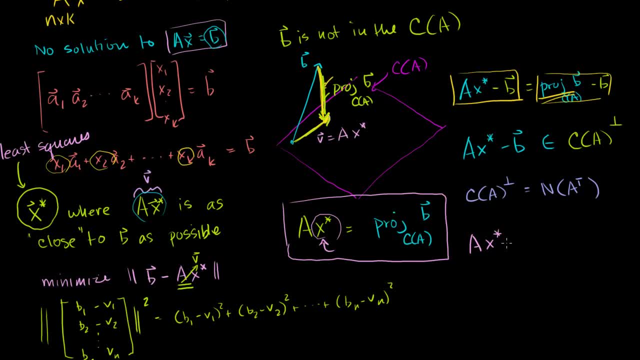 to ax is equal to b. So a times that minus b, minus b is a member of the null space of a transpose. Now, what does that mean? Well, that means that if I multiply a transpose, if I multiply a transpose times- this guy right here. 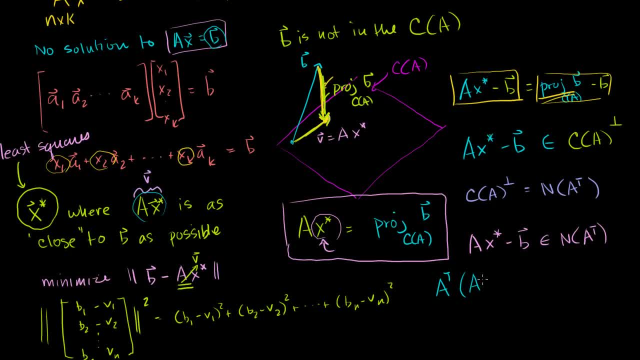 times a, ax star. and let me- I don't want to lose the vector signs there on the x, This is a vector, Don't want to forget that- ax star minus b. So if I multiply a, transpose times this right there. 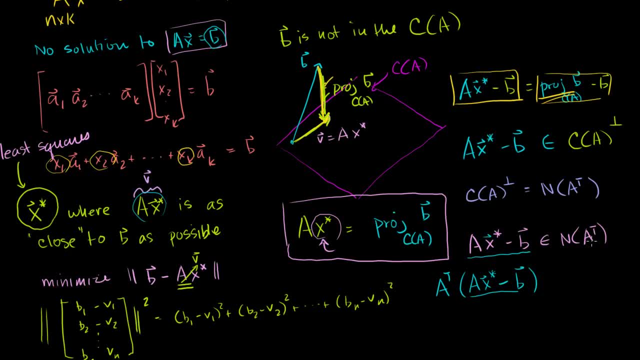 that is the same thing as that. What am I going to get? Well, this is a member of the null space of a transpose, So this times a transpose has got to be equal to 0. It is a solution to a transpose times something is equal to. 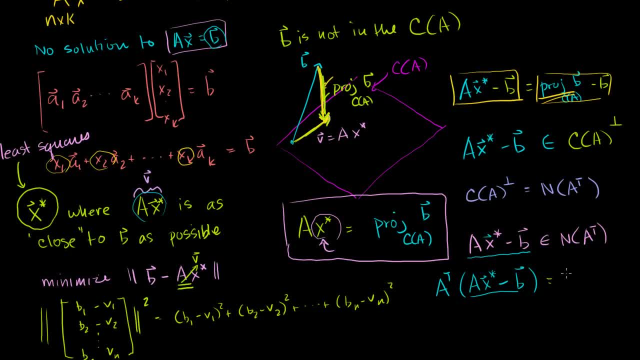 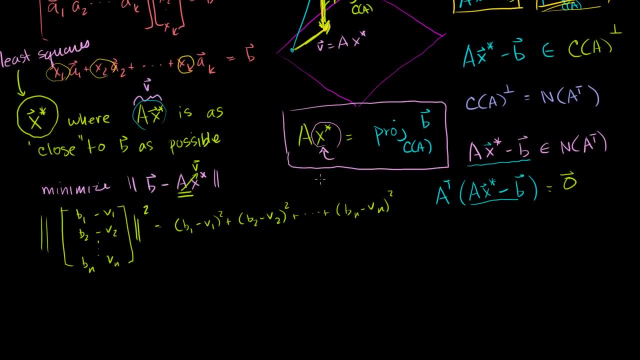 It is a solution to A transpose times. something is equal to is equal to the zero vector. Now let's see if we can simplify this a little bit. We get A transpose A transpose A. times X, star, times X, star minus A transpose B. 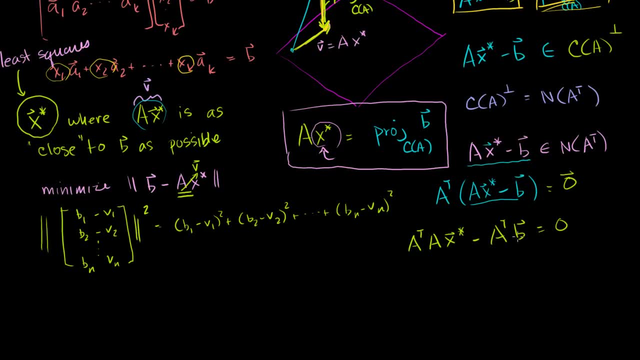 is equal to zero. And then, if we add this term to both sides of the equation, we are left with? we are left with A transpose A times the least squares solution. the least squares solution to AX equal to B is equal to A transpose B. 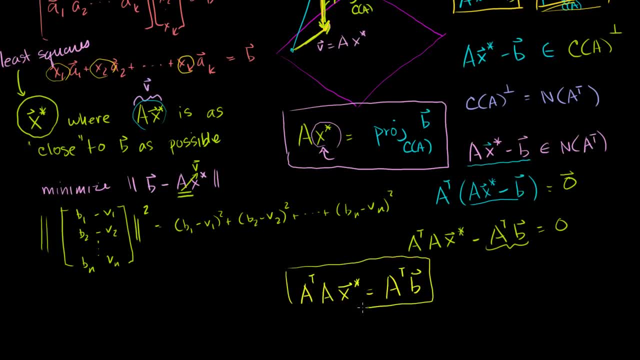 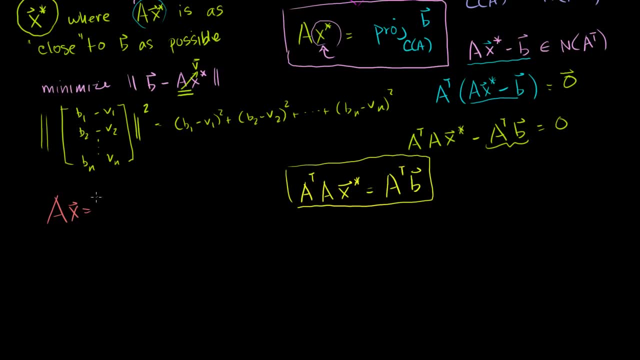 That's what we get Now. why did we do all of this work? Remember what we started with. We said: we're trying to find a solution to AX is equal to B, but there was no solution. There was no solution, So we said: 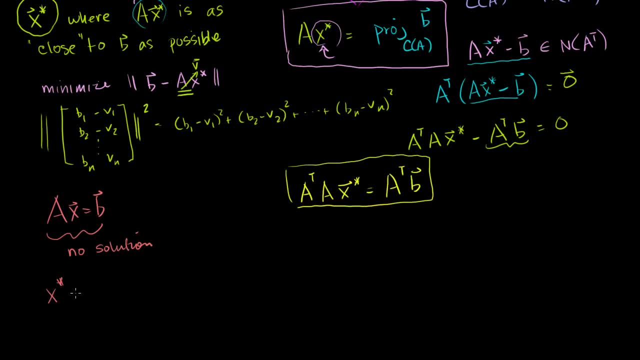 well, let's find at least an X star. let's at least find an X star that minimizes. that minimizes B, that minimizes the distance between B and AX star, And we call that, we call this the least squares solution. 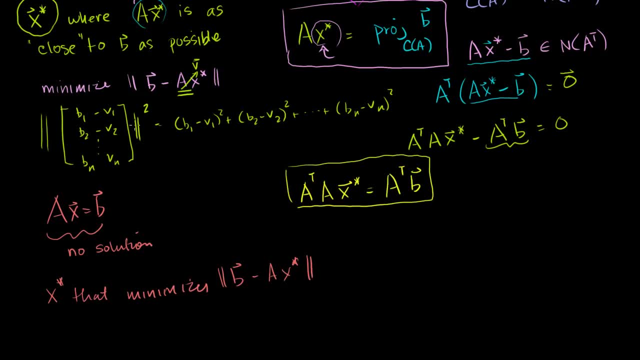 We call it the least squares solution because when you actually take the length, or when you're minimizing the length, you're minimizing the squares of the differences right there, So it's the least squares solution. Now we to find this. we know that this has to be the closest vector. 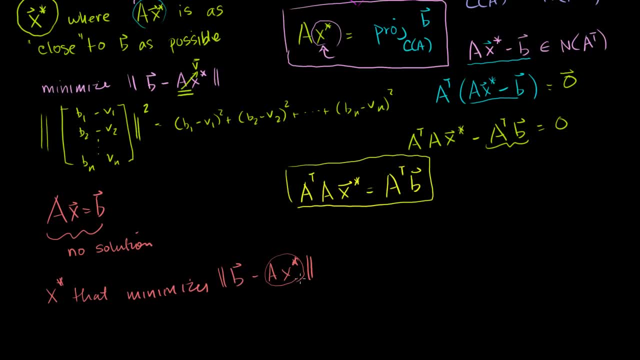 in our subspace to B, And we know that the closest vector in our subspace to B is the projection of B onto our subspace, onto our column space of A, And so we know that we know that A. let me switch colors. 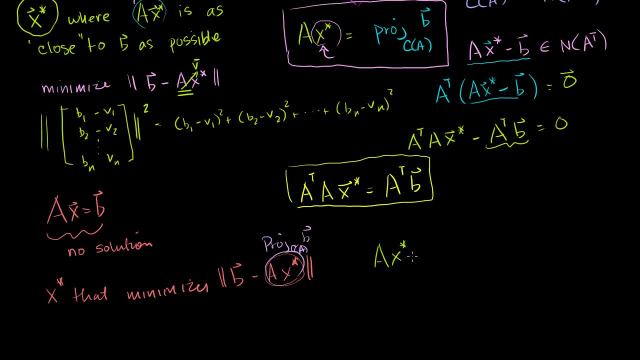 we know that A times our least squares solution should be equal to the projection, the projection of B onto the column space of A. If we can find some X in RK that satisfies this, that is our least squares solution. But we've seen before that this. 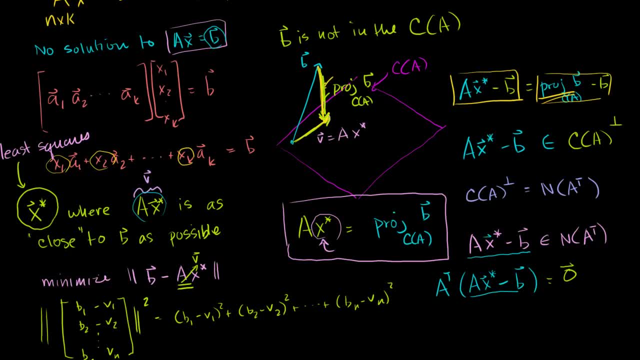 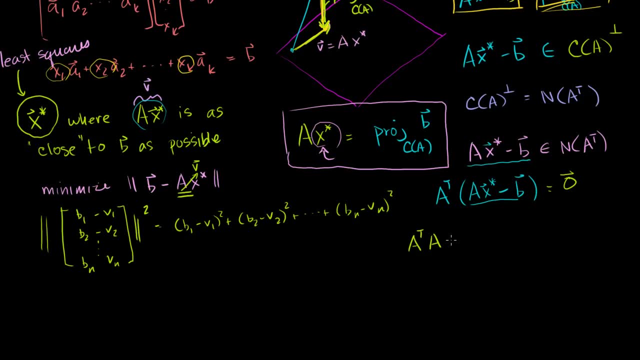 is equal to a 0 vector. Now let's see if we can simplify this a little bit. We get a transpose a. transpose a times x star, times x star minus a transpose b is equal to 0. And then if we add this term to both sides of the equation, 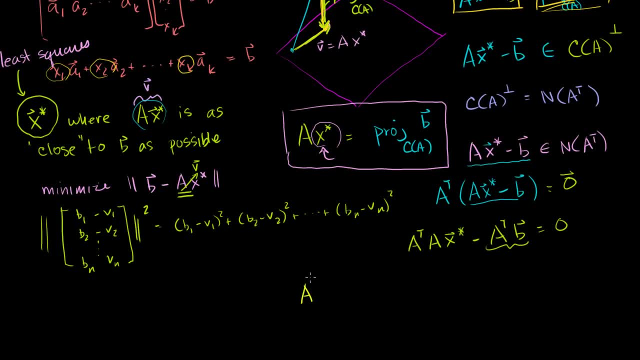 we are left with? we are left with: a: transpose a times the least squares solution. the least squares solution to ax equal to b is equal to a: transpose b. That's what we get Now. why did we do all of this work? 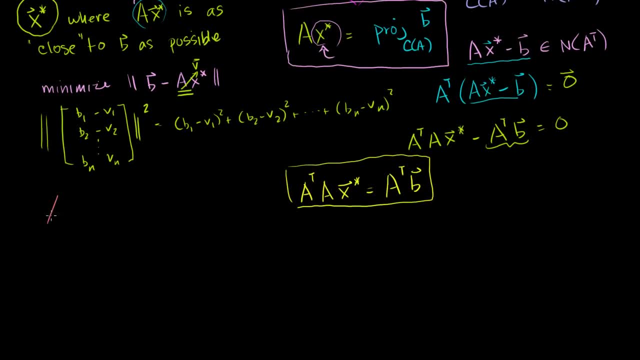 Remember what we started with. We said: we are trying to find a solution to ax is equal to b, but there was no solution. There was no solution. So we said: well, let's find at least an x star. let's at least find an x star. 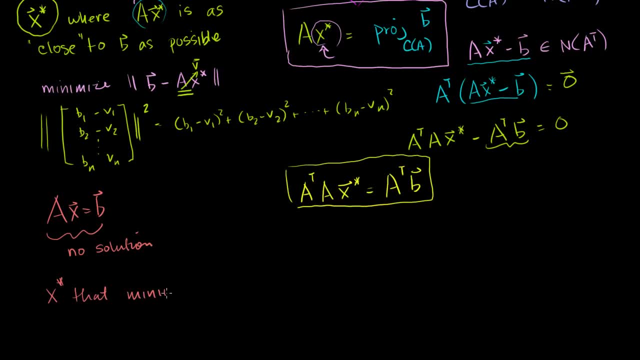 that minimizes, that minimizes b, that minimizes the distance between b and ax star. And we call that, we call this the least squares solution. We call it the least squares solution because when you actually take the length, or when you are minimizing the length, 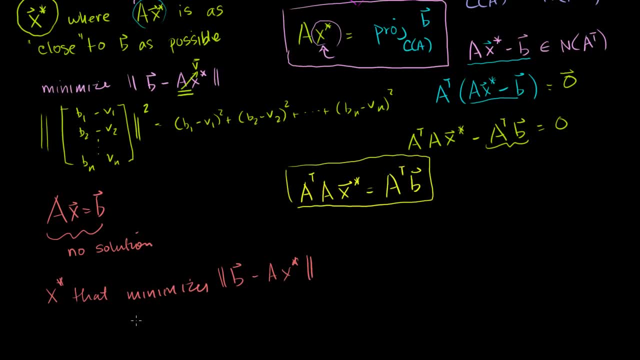 you are minimizing the squares of the differences right there, So it's the least squares solution. Now we to find this. we know that this has to be the closest vector in our subspace to b, And we know that the closest vector in our subspace to b. 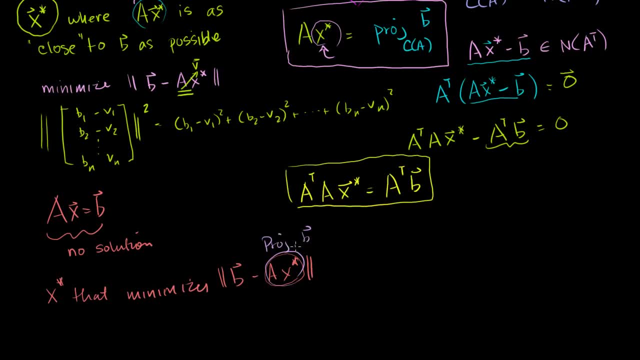 is the projection of b onto our subspace, onto our column space of a, And so we know that, we know that a- let me switch colors- we know that a times our least squares solution should be equal to the projection. 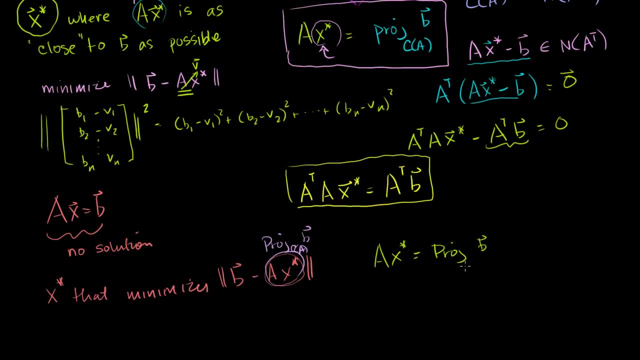 the projection of b onto the column space of a. If we can find some x in rk that satisfies this, that is our least squares solution. But we've seen before that this- the projection b- is easier said than done. as you know, there's a lot of work to it. 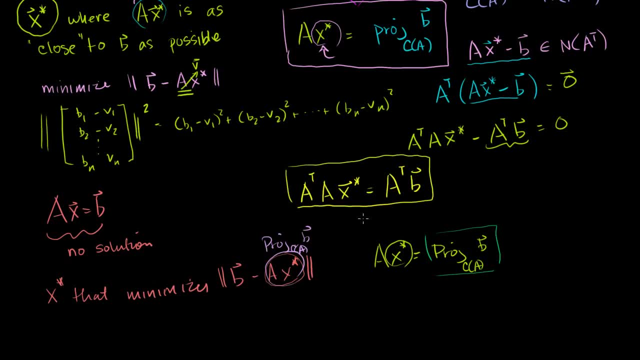 So maybe we can do it a simpler way, And this is our simpler way, If we can, if we, if we're looking for this alternately, we could just find a solution to this equation. So you give me an ax equal to b. 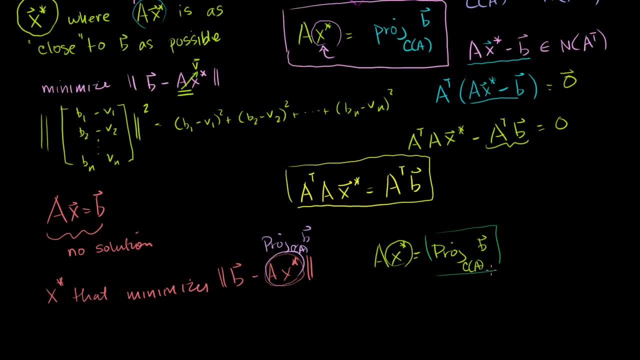 the projection B is easier said than done. As you know, there's a lot of work to it, So maybe we can do it a simpler way. And this is our simpler way, If we can, if we, if we're looking for this. 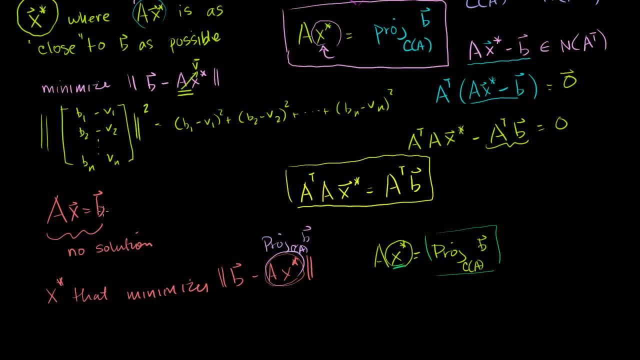 alternately. let's find a solution to this equation. So you give me an AX equal to B. there is no solution. Well, what I'm going to do is I'm just going to multiply both sides of this equation times A- transpose. 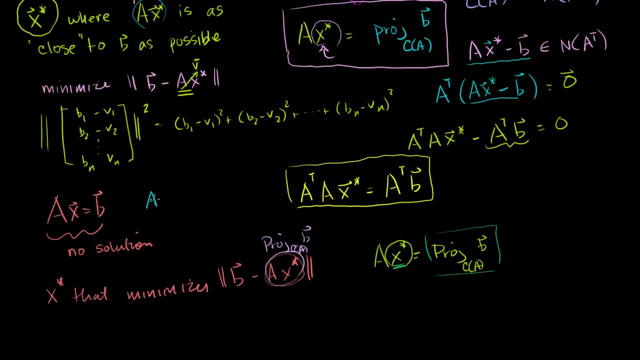 If I multiply both sides of this equation by A transpose, I get A transpose times AX. AX is equal to A transpose. now I want to do that. the same blue A. no, that's not the same blue A transpose B. All I did is I multiplied both sides of this. 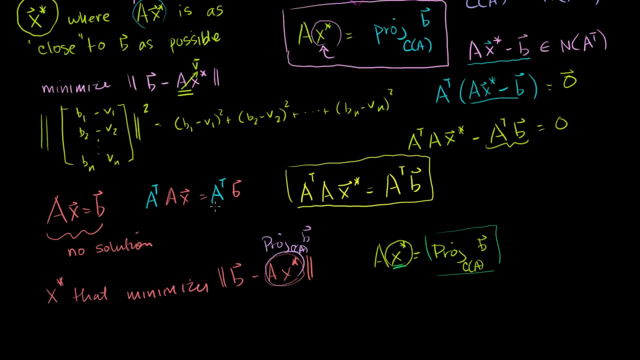 Now, this solution, this solution is not going to be the solution to this equation, will not be the same as the solution to this equation. This right here will always have a solution, and this right here is our least squares solution. So this right here is our least squares solution. 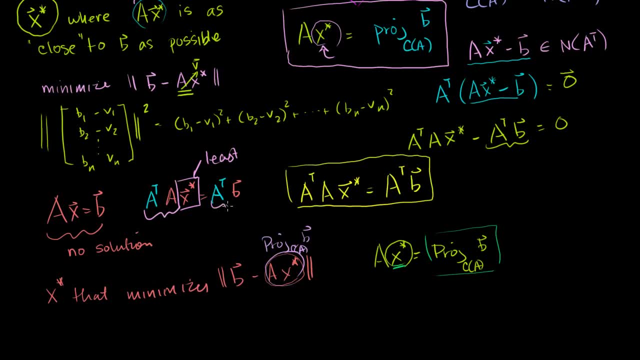 And notice: this is some matrix, and then this right here is some vector, This right here is some vector. So as long as we can find a solution here, we've given our best shot at finding a solution to AX equal to B. 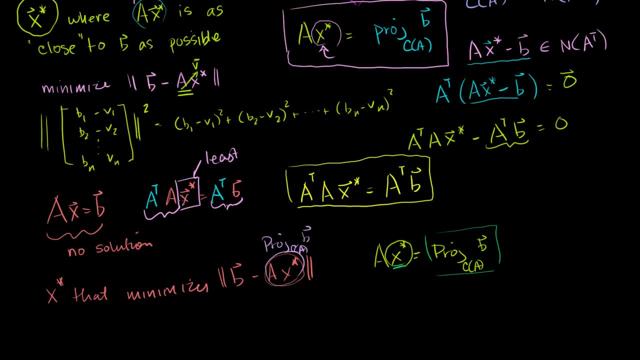 We've minimized the error. We're going to get AX star and the difference between AX star and B is going to be minimized, So it's going to be our least squares solution. It's all a little bit abstract right now in this video. 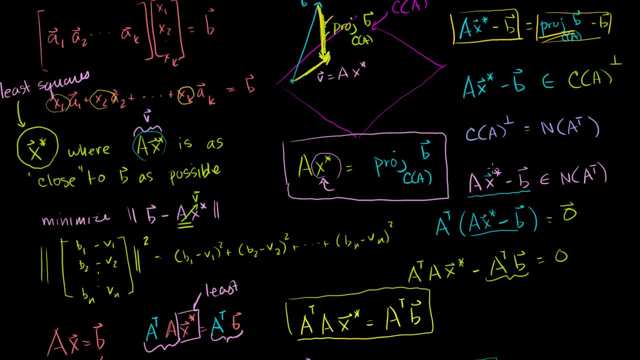 but hopefully in the next video we'll realize that it's actually a very, very useful concept. 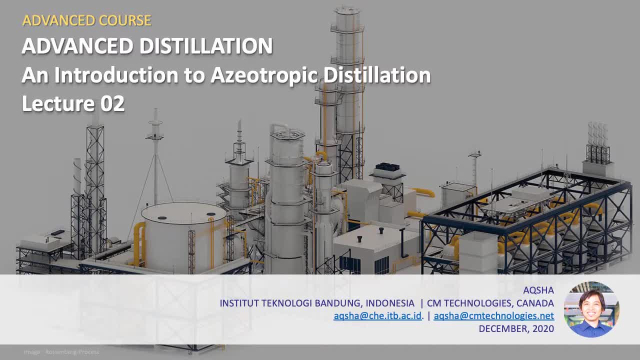 Hello everyone, this is Aksa and I welcome you into the lecture 2 of the introduction to azeotropic distillation. So previously we've just learned about what is azeotrope and how it forms, and so on. In this particular lecture we're